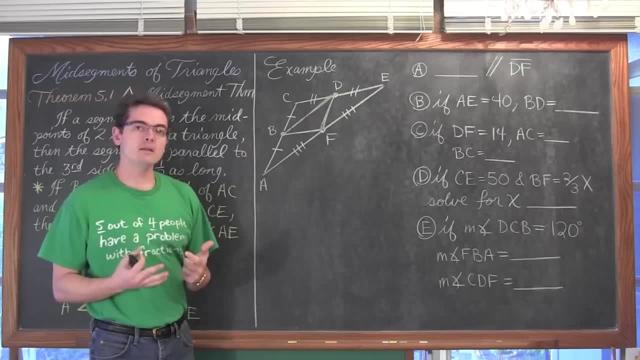 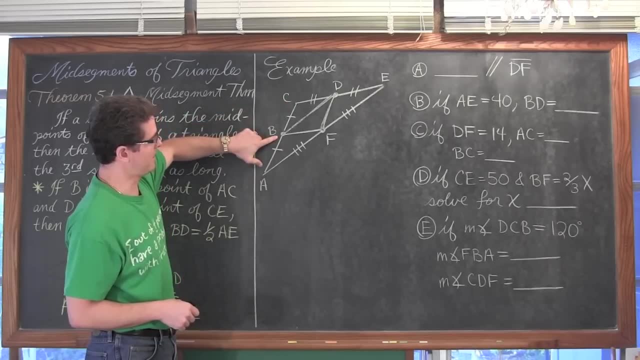 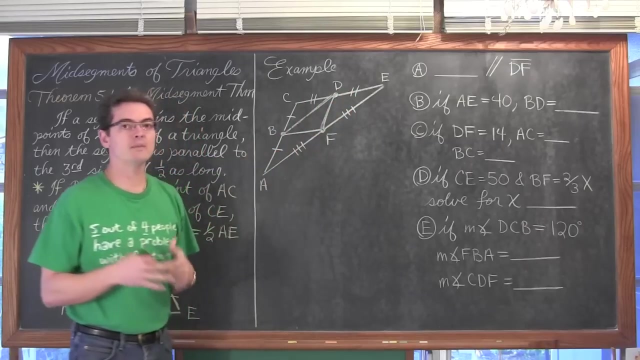 have to say that these points are mid points. They are in that. you can find them in the diagram: These two tick marks showing that BC is congruent to BA. The same thing over here with the tick marks at CD and DE, You know, stating that these segments are congruent. 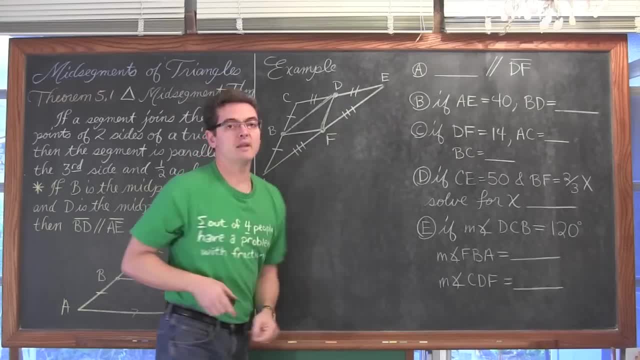 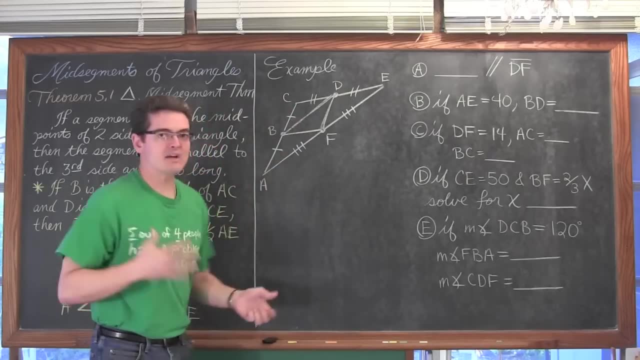 that is what a mid point does: It takes the segment and cuts it in half. Let's start taking a look at some of these examples. Ok, So first of all, we are just going to try to identify the mid point and that segment that is parallel to it. So I have a blank here and it is parallel. 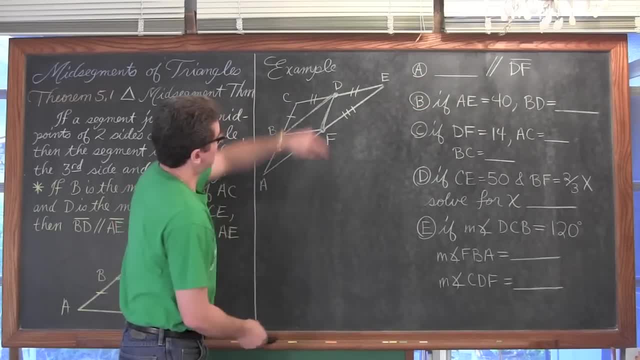 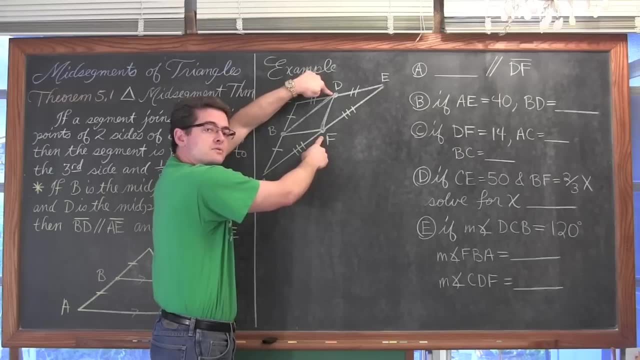 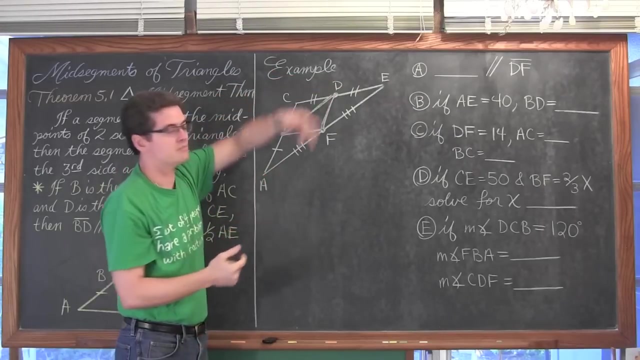 to DF. Well, let's find DF. DF is a mid point connector and therefore that segment connecting the mid points of two sides of our triangle is going to be parallel to the third side, The side that isn't being cut in half by the mid point Connector segment. So if this 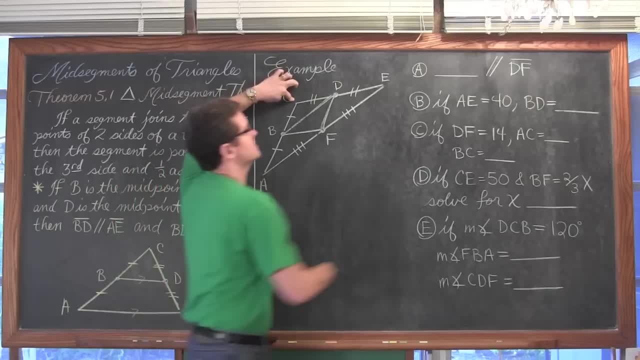 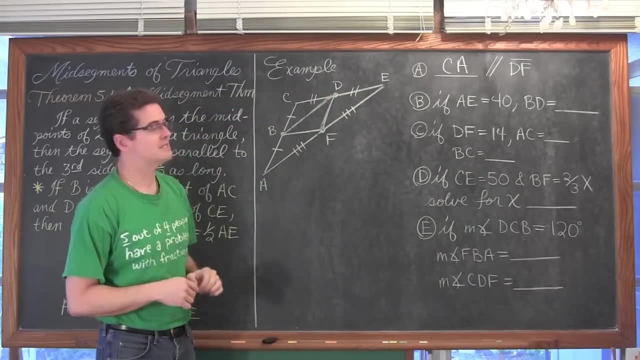 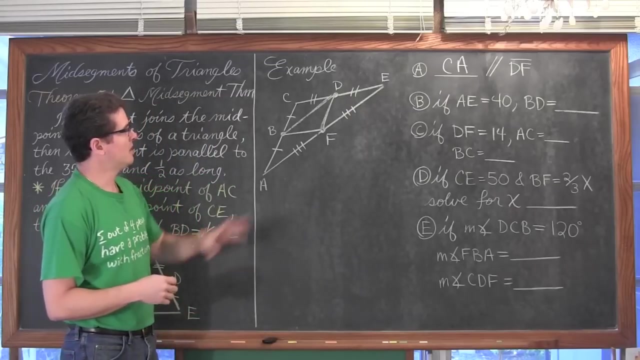 is DF. this is going to be parallel to CA. So there is our answer to part. CA is parallel to the segment connecting the mid points of DF. I have these examples. They don't necessarily tie into each other, They just all use this diagram. So one answer. 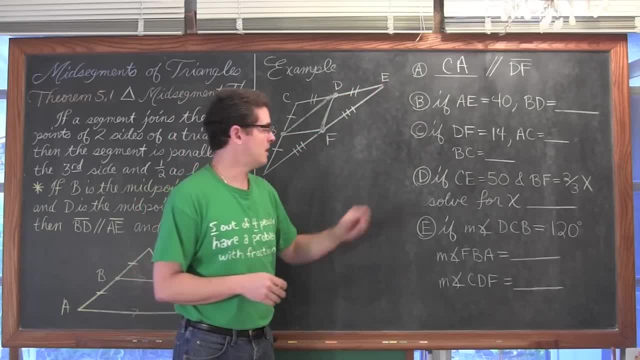 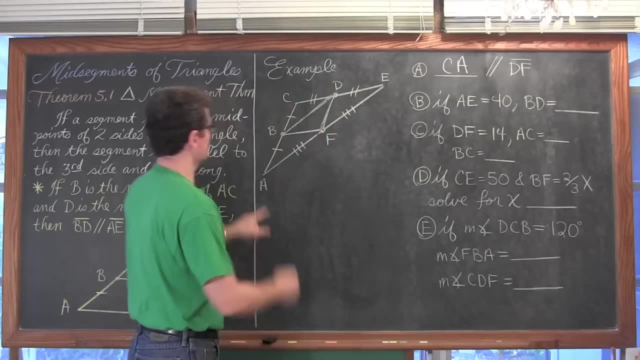 from one of these parts may not necessarily carry through to the other portions of this example. Just be aware of that. Well, we have here that says AE is equal to 40. So AE, the entire length of the segment of a triangle, is equal to 40. Well then, that means that 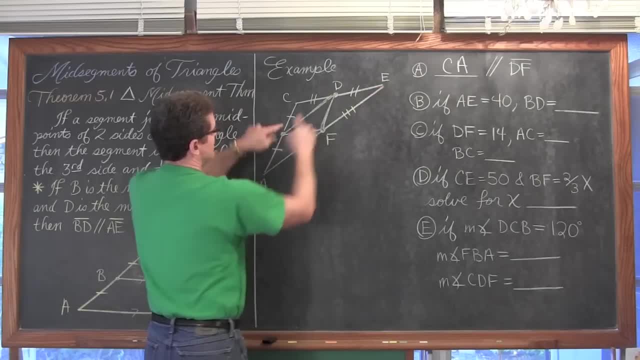 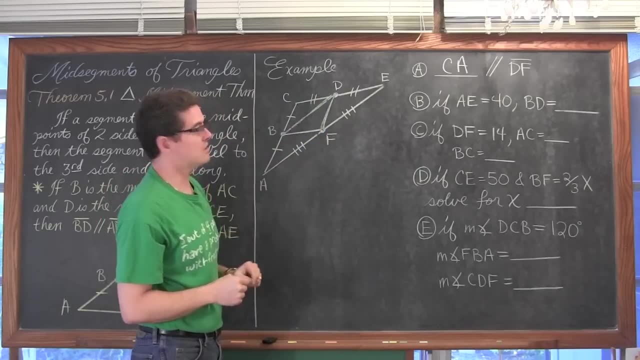 BD. Ok, let's see here We have AE and we have BD, again connecting mid points of the other two sides of the triangle. So this length is going to be half. This segment connecting the mid points is going to be half of the third side, which means it is going to be: 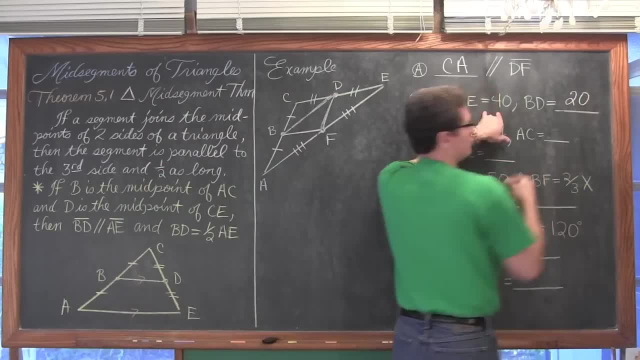 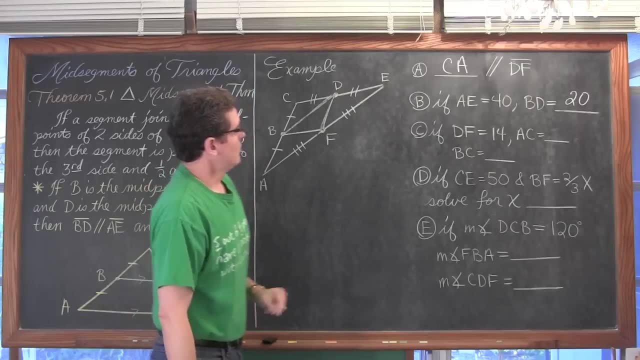 half of 40,, which is equal to 20.. When you take half of a number, you are simply dividing it by 2, and 40 divided by 2 is equal to 20.. Well, let's see what else we have. We have: 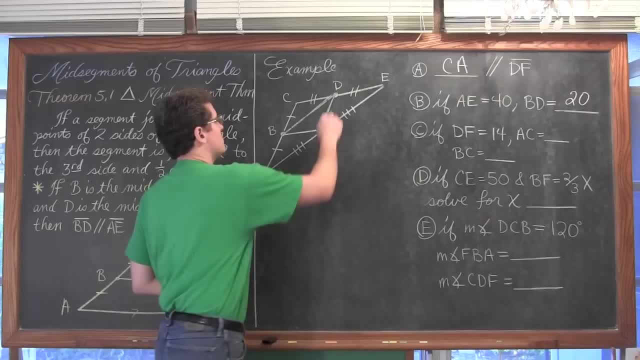 DF is equal to 14.. So let's see what else we have. We have DF is equal to 14.. So we have DF is equal to 14.. Let's just temporarily write that in there so I don't forget what. 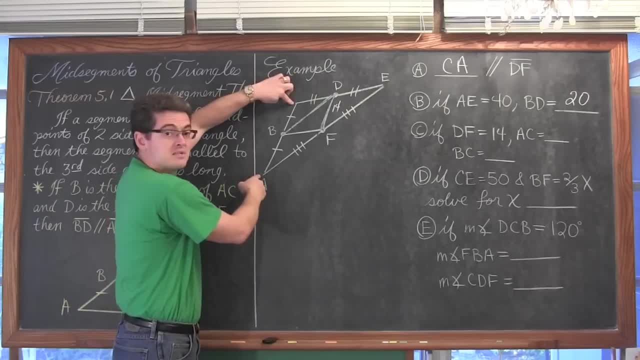 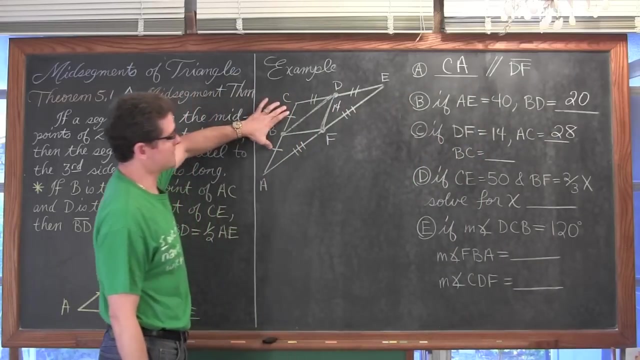 I am doing here. We are being asked for the length of AC, So I have given us the length of the segment connecting the mid points. The side which that is parallel to is going to be twice as long. 4 times 2 is equal to 28.. Alright, so this entire length is 28.. 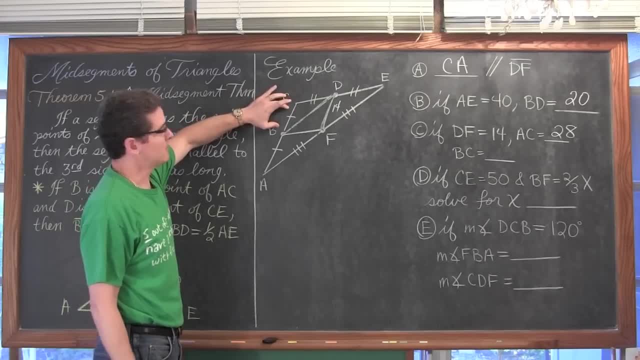 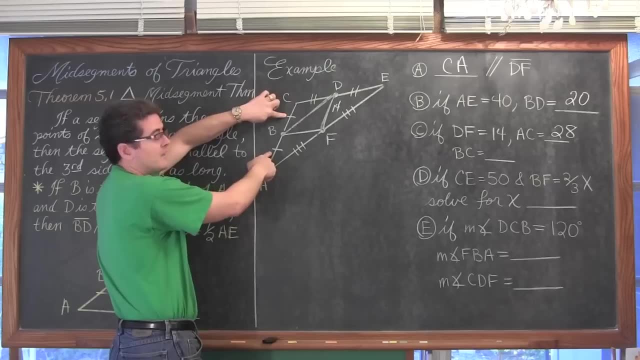 Well, what is BC? Well, there is not a congruency mark here. You know, this length is 14 and all I am stating is that these two parts are congruent. So you might already know the answer is going to be 14, but just for argument's sake, we 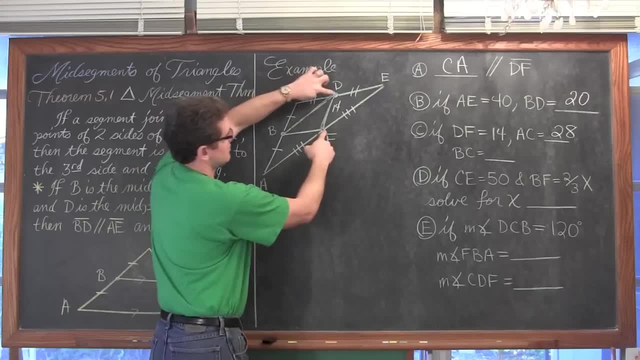 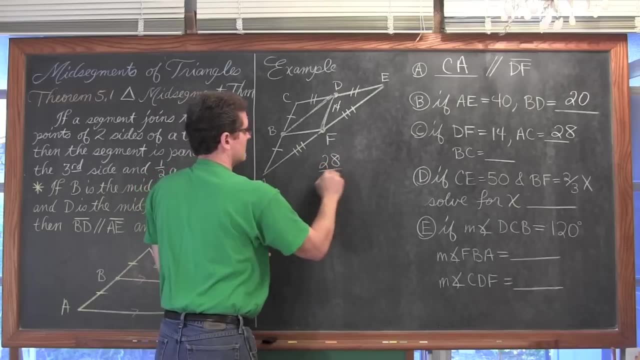 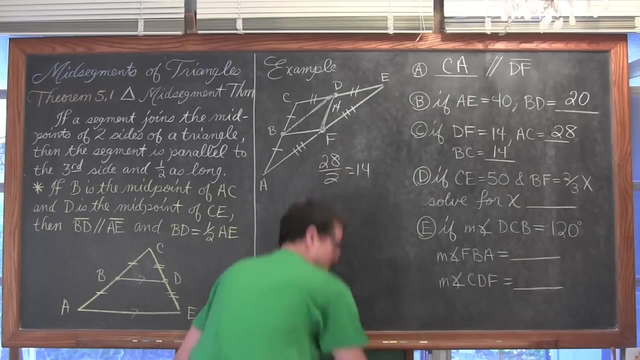 have the 28, that is double 14.. Ok, 28 is being cut in half by the mid point and half of 28 is equal to 14.. Let me move that board so it stops rattling. Ok, well, we got that answer. Let's get on to part D. Part D says that we have got if. 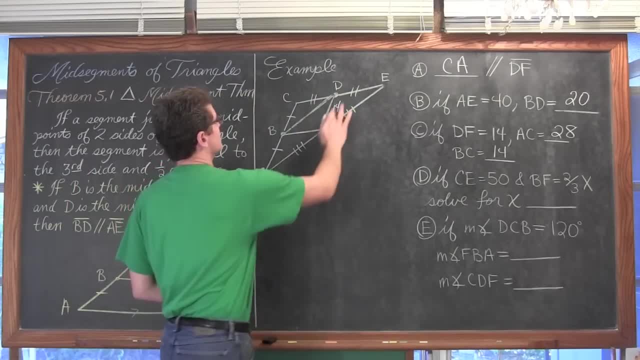 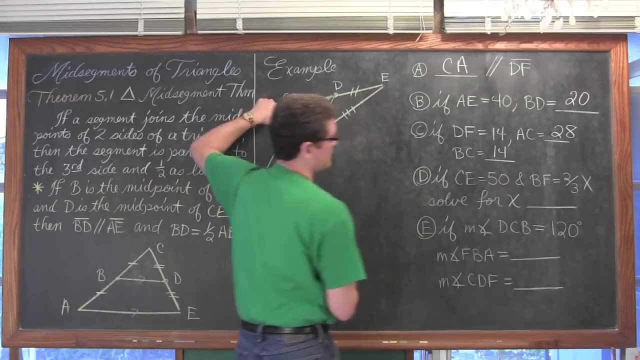 CE is equal to 50.. So if CE- Let me take this out of here, We are not using that anymore- This entire length is equal to 50 units. If CE is equal to 50, then BF is equal to 2 thirds. 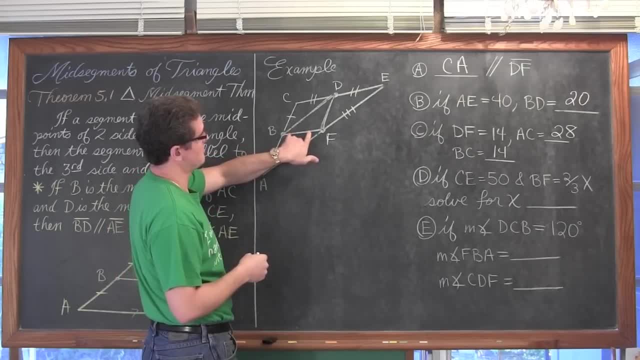 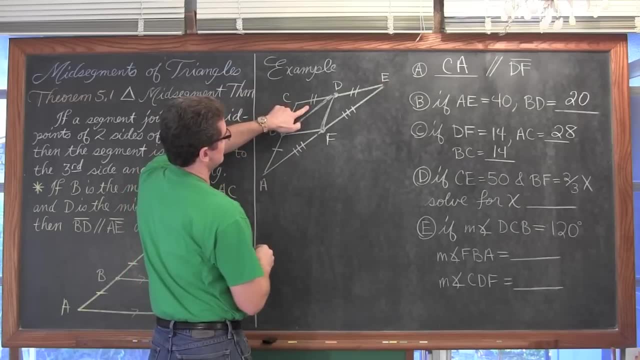 X. Ok, so this segment, This segment connecting the mid points, is equal to 2 thirds X. Ok, so this segment, This segment connecting midpoints of these two sides, is half of this length. So I can take the 50 which we are. 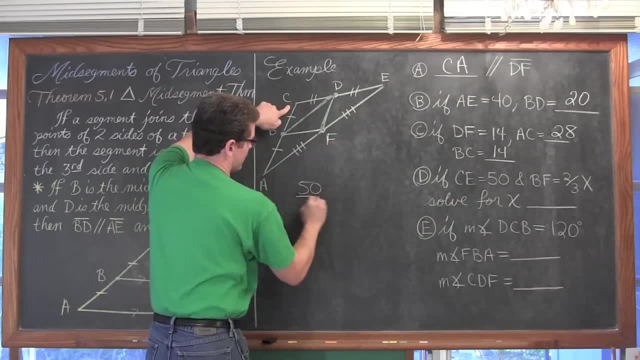 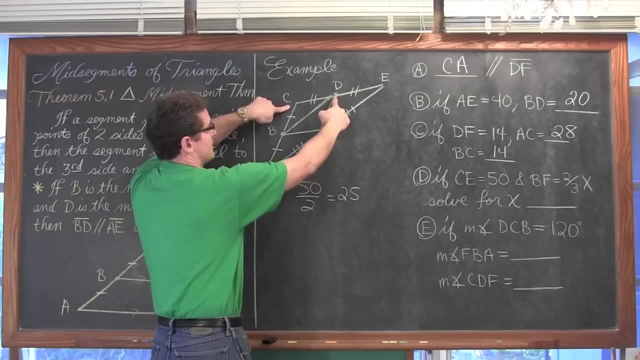 told is the length of CE. I can divide that by 2 and get 25.. So this segment is now an entire length of 50, but if I cut it in half I get 25.. BF is half of that overall length. 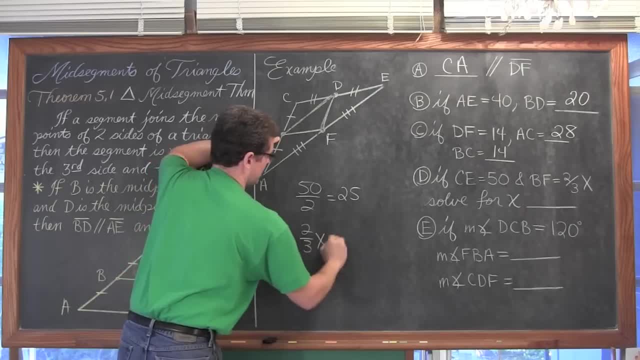 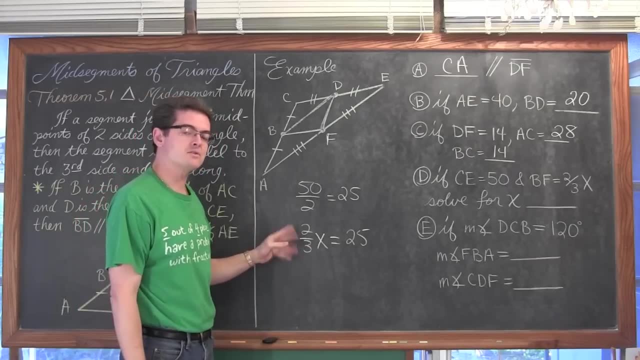 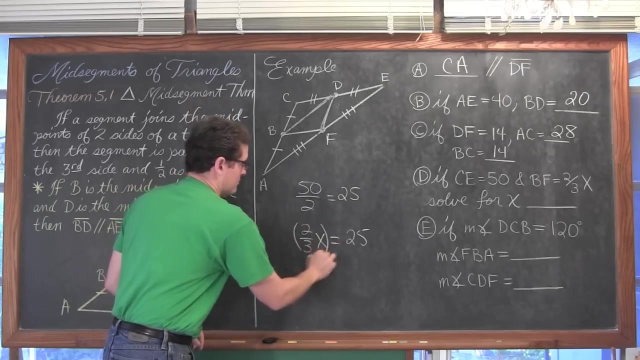 So BF, which is 2 thirds x, is equal to the length of 25.. Alright, so some of us are not always the most comfortable with fractions. We are going to take care of that by multiplying both sides by the reciprocal. So if you have a fraction, you can move that fraction to the 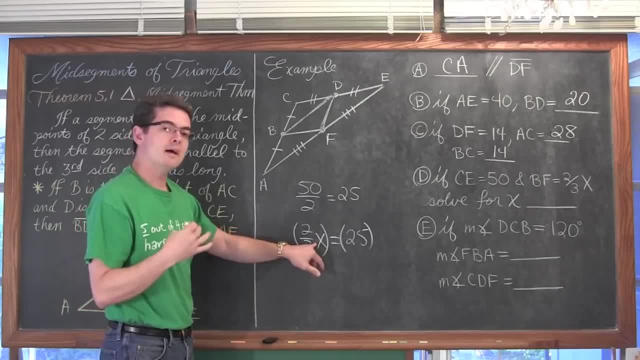 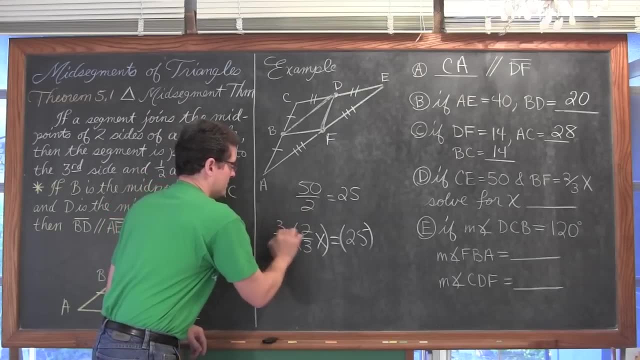 other side of the equation. We are trying to undo that multiplication of 2 thirds. We want to do the inverse math operation and that is multiplying by 3 over 2.. Well, 3 times 3 is 6.. 2 times 3 is also 6 times x. Now hopefully we understand. 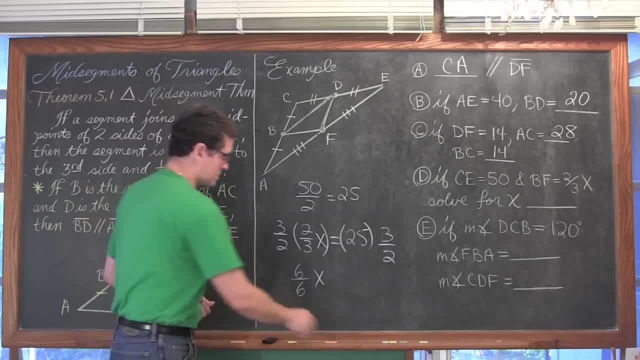 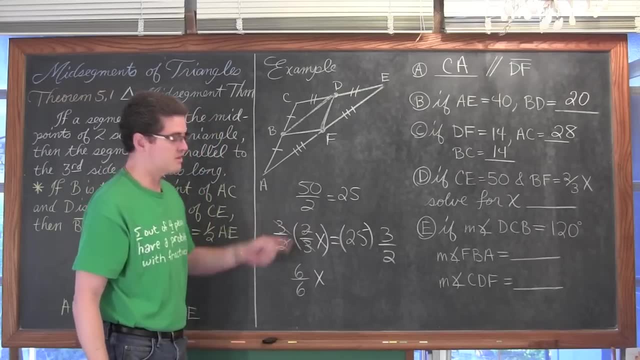 that 6 divided by 6 is going to be equal to 1.. Or I could also come up here and take these 3's and cancel them out. Take the 2's and cancel them out. We can see, with all that cancellation, through the multiplication and division, that this 6 divided by 6 is just. 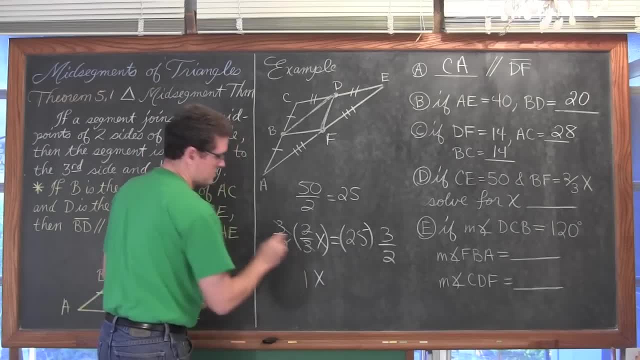 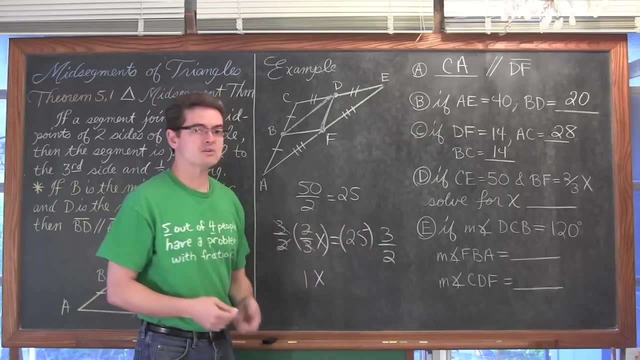 going to be 1.. So I am going to save a little space- Subtitles by the Amaraorg community space- and just write that 1 there. Now, over here, I have 25 times 3 over 2.. Well, when you start doing math with fractions, remember that you might want to just make every single factor. 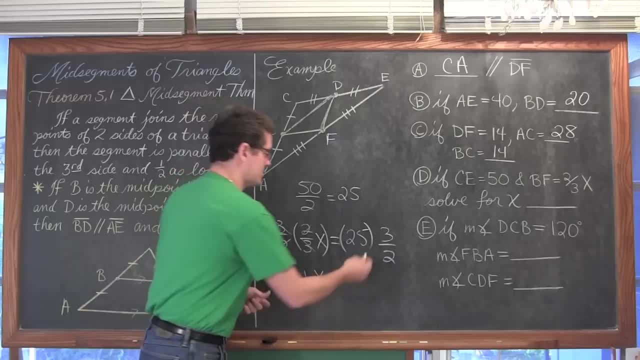 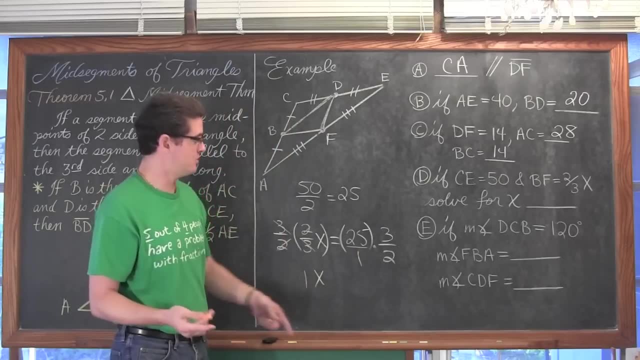 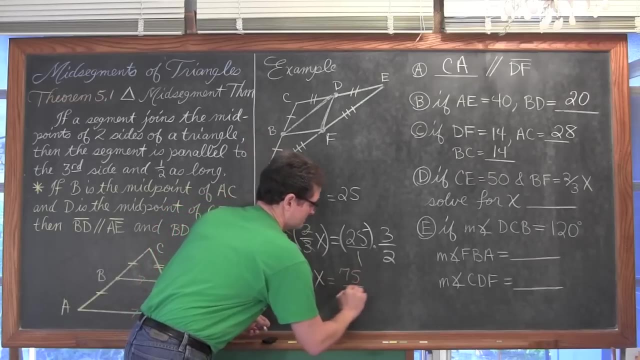 every single term, every single number look like a fraction. So we are going to take this 25.. We are going to put it over 1 and multiply straight across. Now we can do 25 times 3, which is 75, and divide that by 2.. 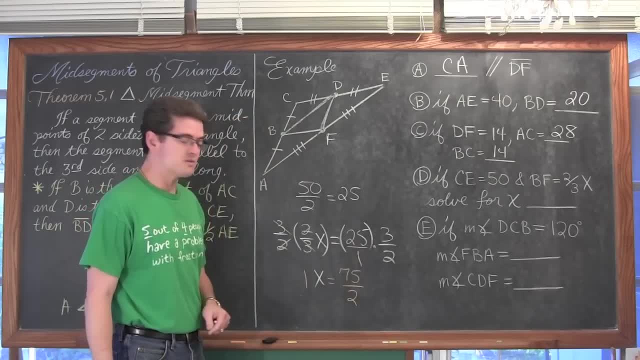 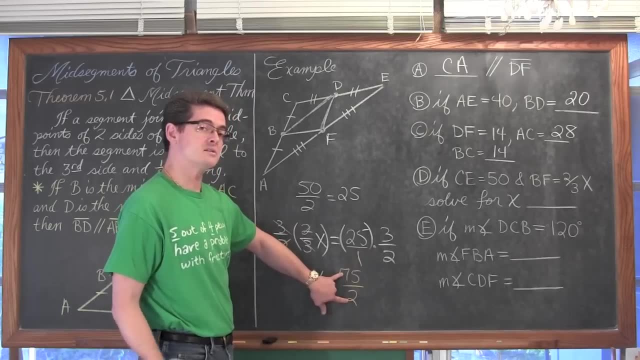 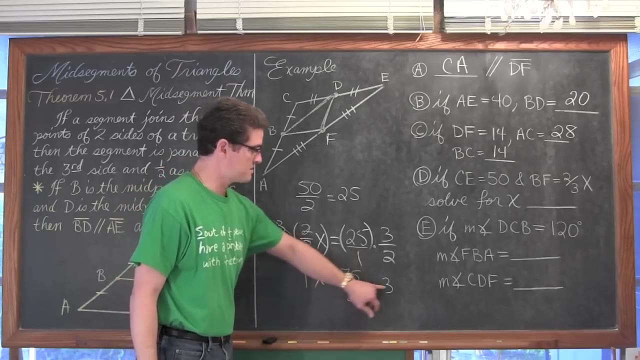 And we can leave this as 75 divided by 2.. We can also actually do the division and make this a mixed fraction. So 7 divided by 2 is 6.. So we are going to have 3, or- excuse me, I was thinking of the answer- 7 divided by 2 is 3.. Now, 2 times 3 is equal to 6, leaving. 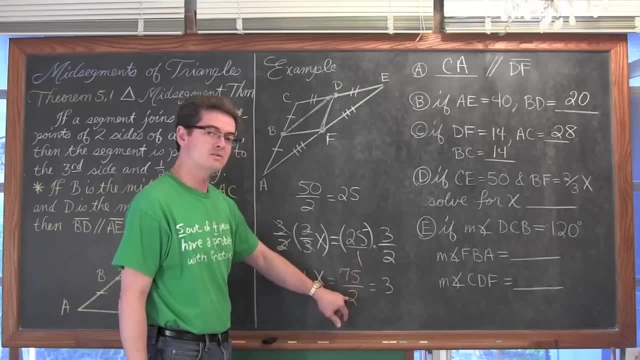 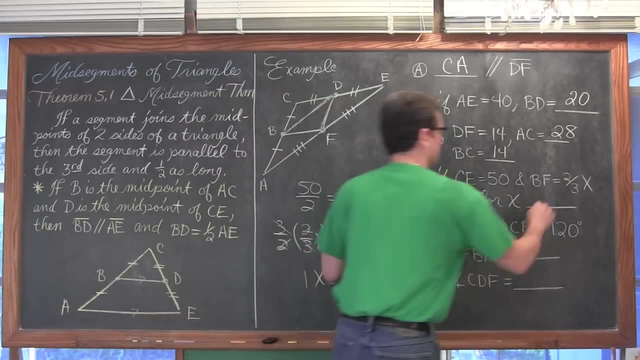 us with a remainder of 1.. Well, 15 divided by 2 is going to be 7.5.. So our final answer here is 37.5.. And that is our answer for x. Over here we have our answer for x. We are. 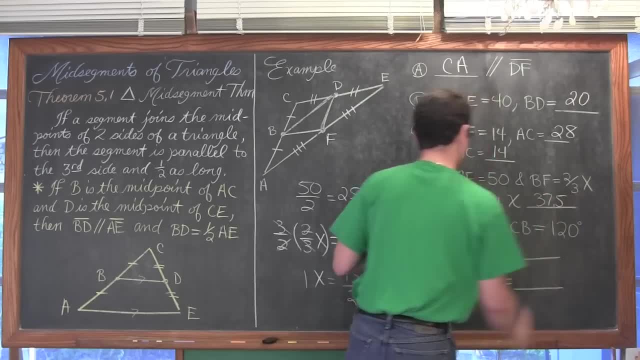 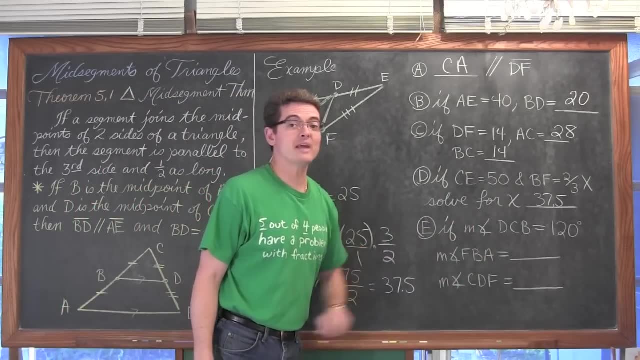 going to have our answer for x over here on part d. Ok, Let's clear off this board a little bit so I have some room and make sure that I don't make a big mess as I try and answer this last part. Be right back, Alright, We are almost done with this example. 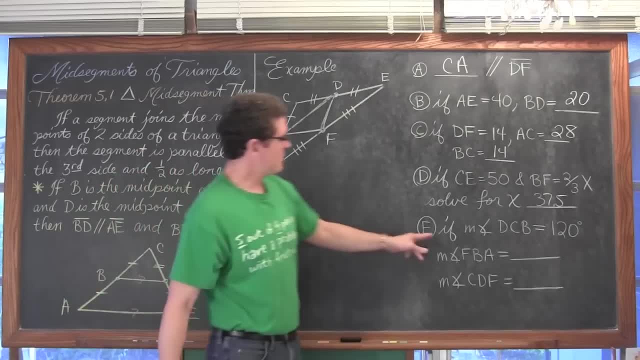 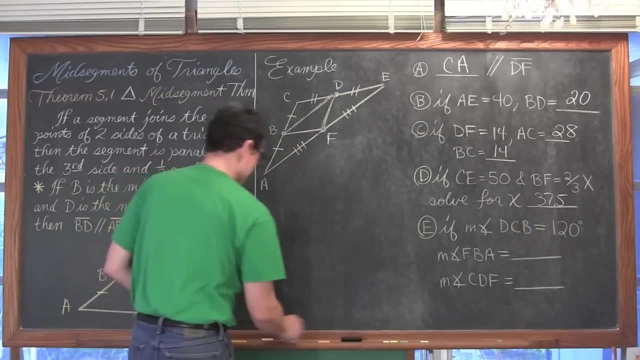 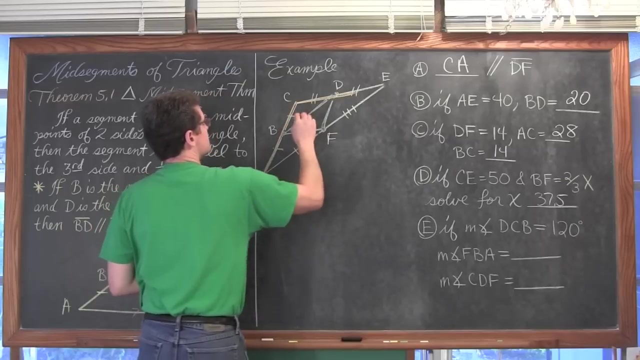 and this diagram, So I am going to start drawing all over it. We have here. in part e it says the measure of angle dcb is equal to 120 degrees. So let me get some orange chalk here. dcb, So this angle is equal to 120 degrees. And now it is saying: what is the measure of angle? 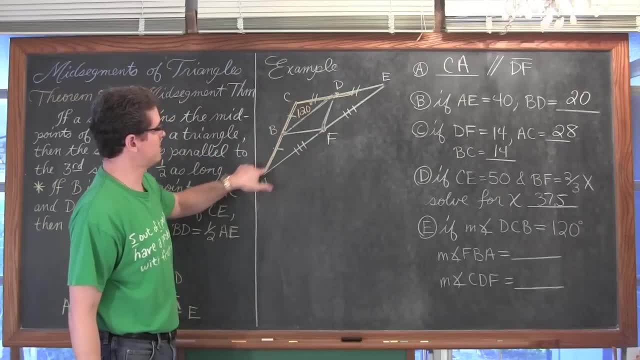 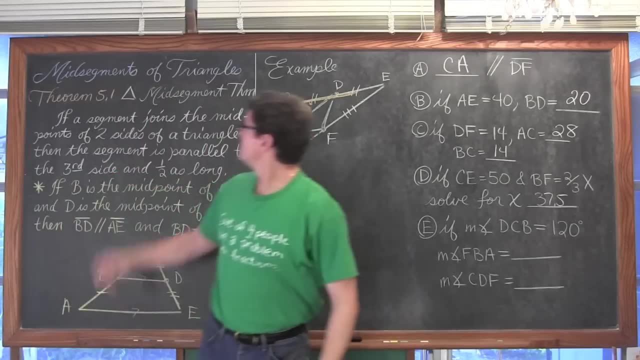 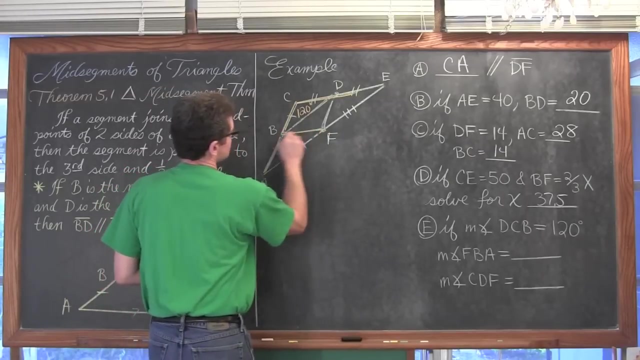 fba. Well, fba is here. Now fba: the first two points that are making this angle. those are a segment which connects the midpoints of a triangle, So that means that this segment of bf is going to be the angle of angle bf. So that means that this segment of bf is going 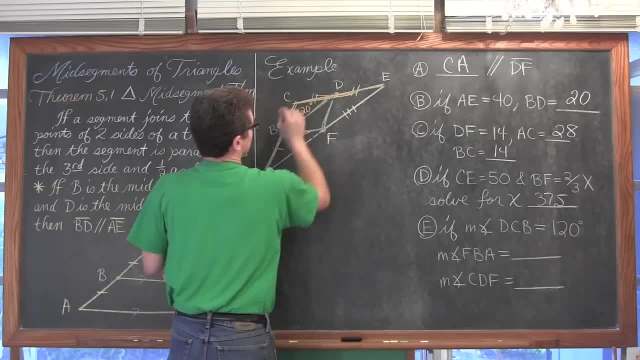 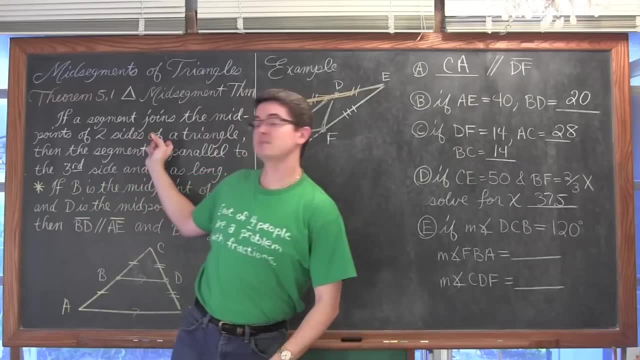 to be the angle of angle bf. So that means that this segment of bf is going to be the parallel to this line segment and we can refer to line segment cd or ce. These are going to be parallel as part of this theorem. So we have two parallel lines being cut by. 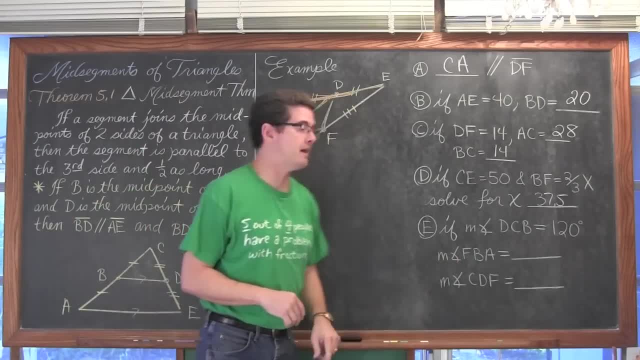 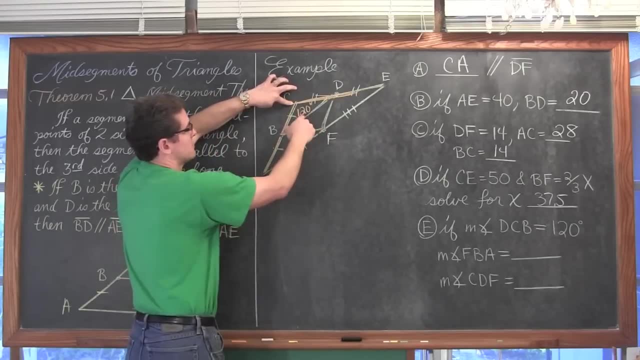 a transversal and that is going to help us answer the measure of angle fba, This intersection. right here are two parallel lines being cut by a transversal. This 120 degrees is at the hand corner. Well, FBA is talking about this angle right here, which is again in the lower. 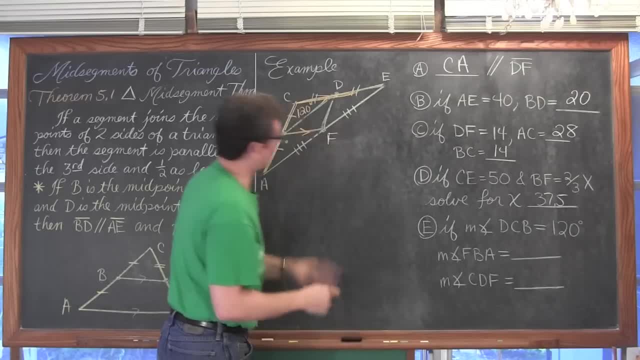 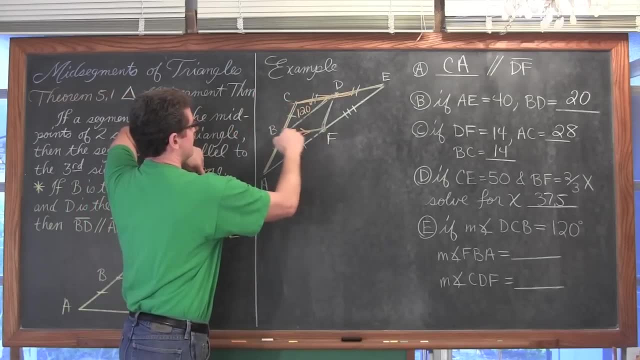 excuse me, I just said the wrong answer. Well, that is ok. Let me correct that. The 120 is in the lower right hand corner. I think I said lower left, So angled FBA is also in the lower right hand corner. So these are corresponding angles, Angles, which are both. 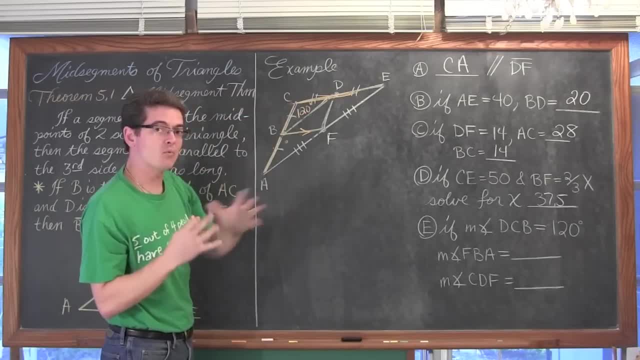 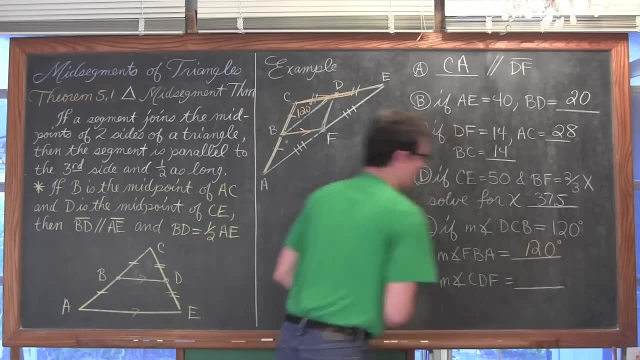 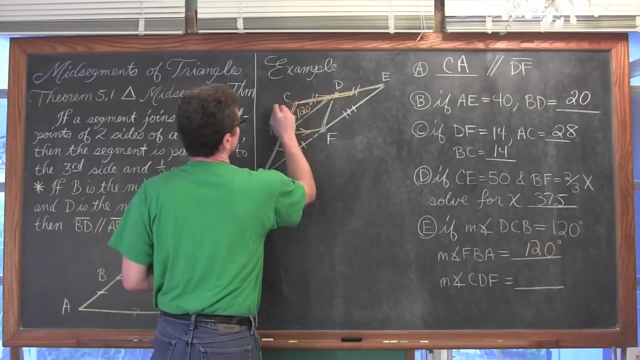 in the lower right hand corner are both in the same relative position, are going to be congrowing. Angle FBA is equal to 120 degrees. Ok, now we are being asked down here for angle CDF. Well, we have again. let's see here CDF. Well, let's focus on these segments. This. 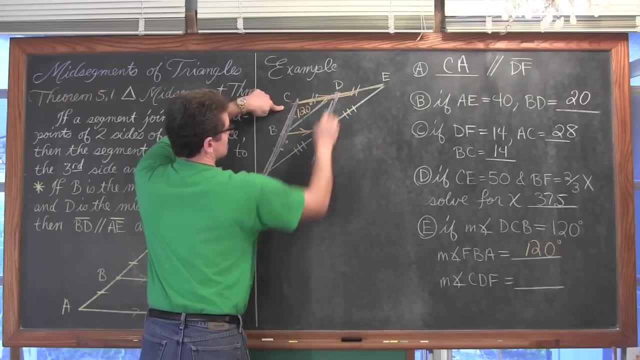 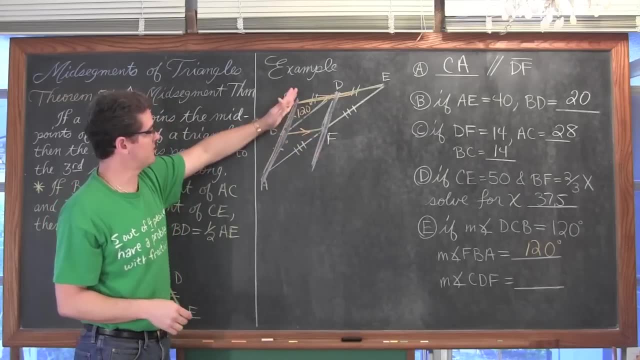 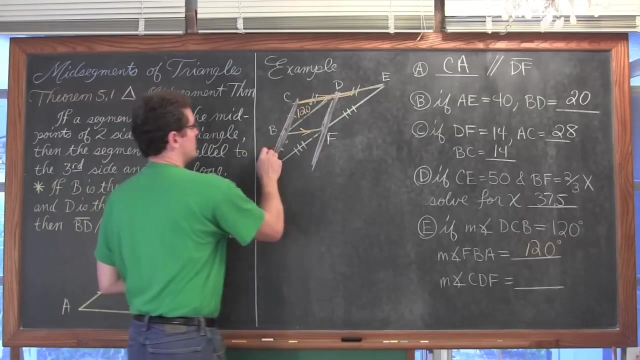 one. right here We have this segment connecting the midpoints, the segment of DF. These two lines are going to be parallel: This side of the triangle and this segment that is connecting the midpoints of those sides. So these are going to be parallel. 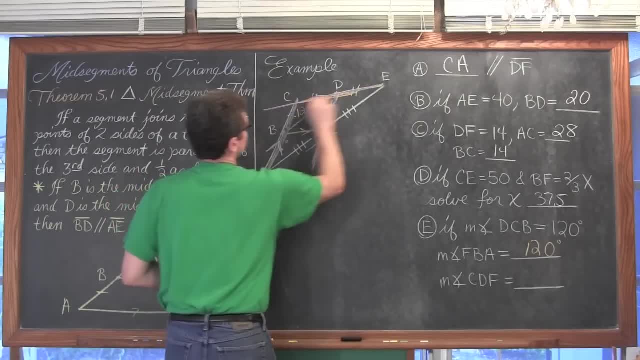 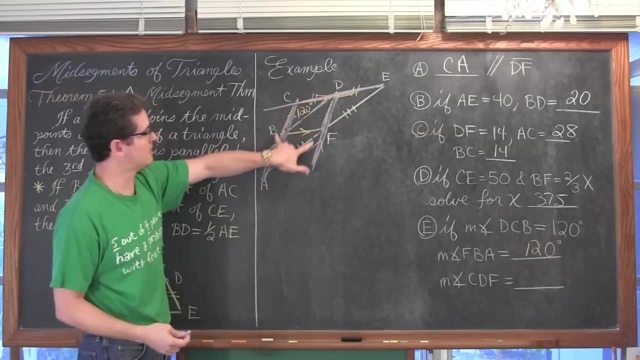 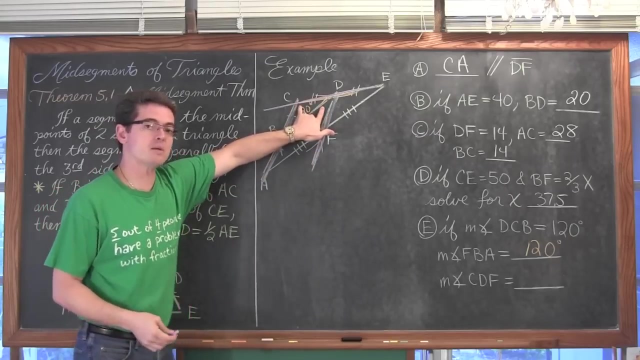 another set of parallel lines being cut by a transversal- Hopefully remember that same side- interior angles are going to be supplementary. when two parallel lines, the side of the triangle and the parallel segment which connects the midpoints, those same side interior angles are going to be supplementary. So we have 120 degrees plus. excuse the noise there. 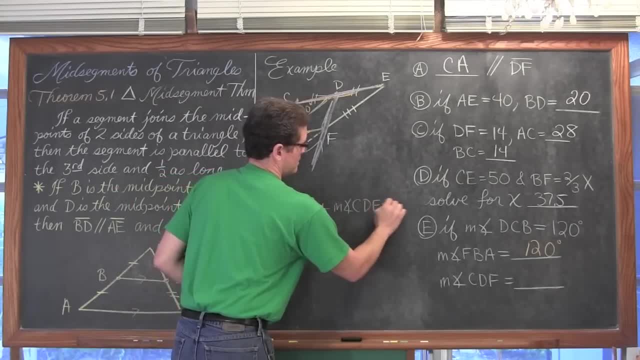 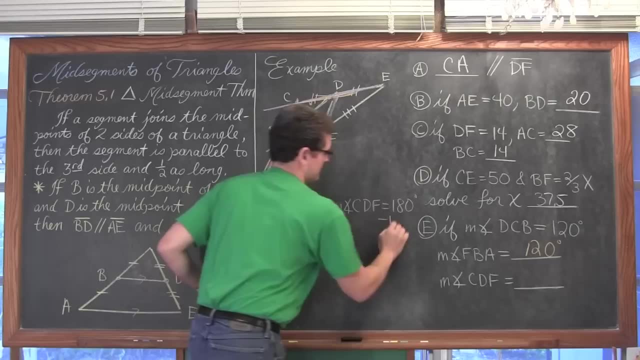 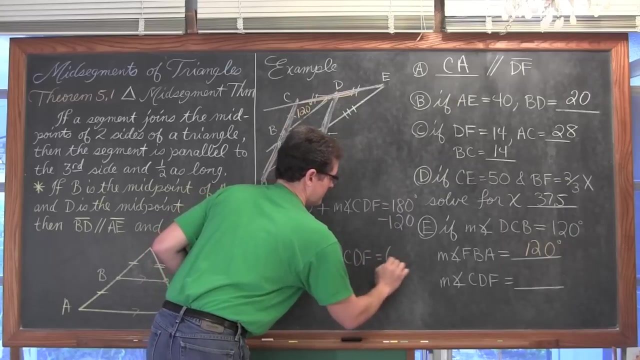 the measure of angle CDF is going to be equal to 180 degrees. We are going to subtract both sides by 120 and get the measure of angle CDF is equal to 60 degrees. Let's get on to our next example, Dr B, Next example: 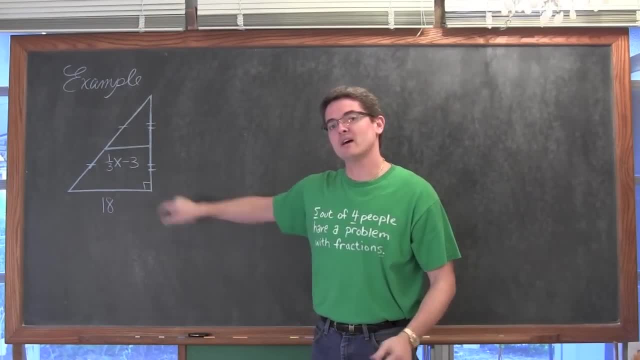 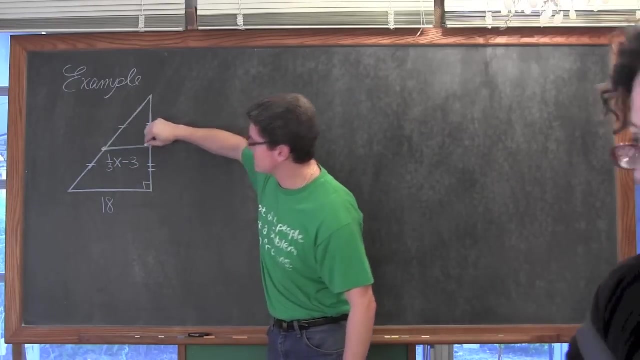 Dr B, We have another right triangle. now We have a segment connecting the midpoints of our triangle. I want to use this information to solve for x. I am not going to need a bunch of coordinates, so I left the variables off of here. Just a right triangle, a segment. 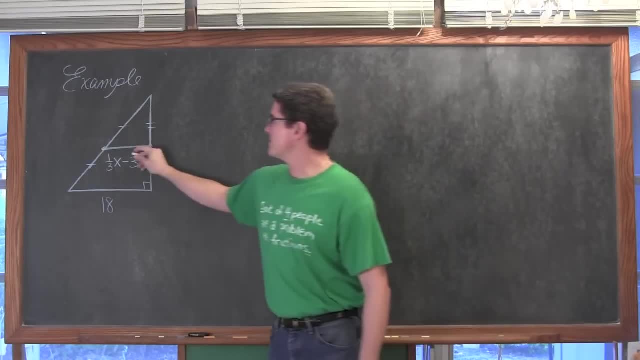 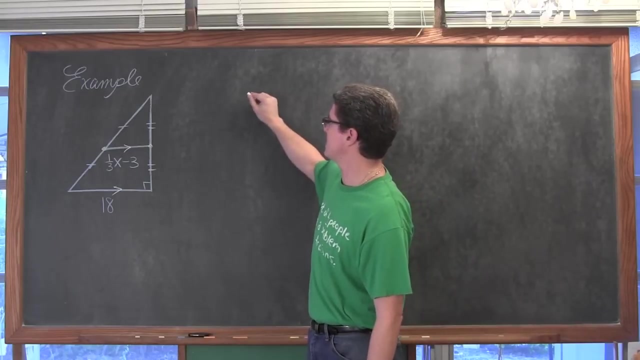 connecting the midpoints of two sides, and thus this segment is going to be parallel to the third side and half of it is left. If I want to use this information to figure out what the length of x is, there are a couple ways I can set this up. I can say that 2 of the segments which connect the midpoints is 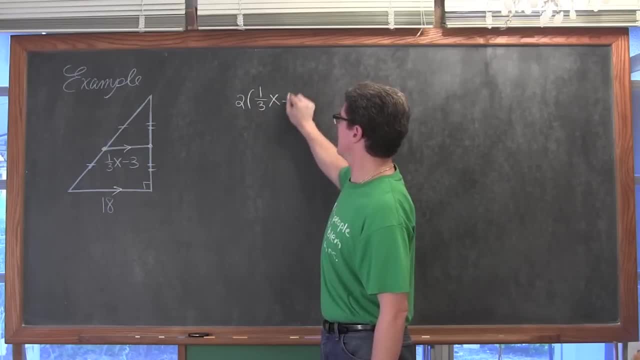 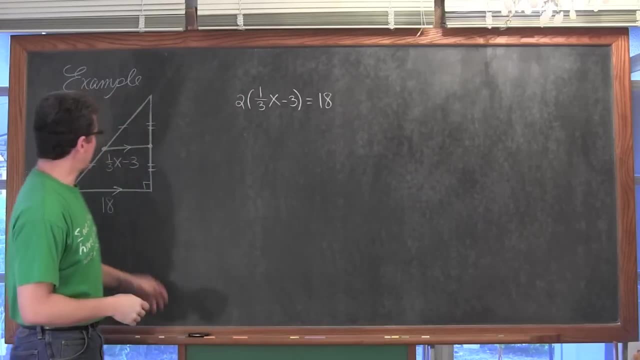 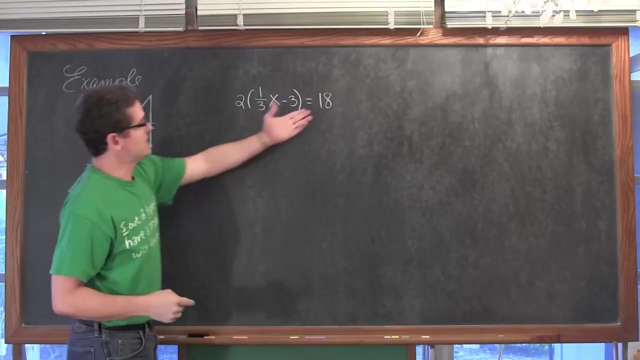 equal to 2 of those. 2 times 1 third x minus 3 is equal to 18.. I could have started off setting up my problem this way, or I could have said: this segment is equal to half of the side of which it is parallel to, and just set it equal to 18.. So let's go ahead and 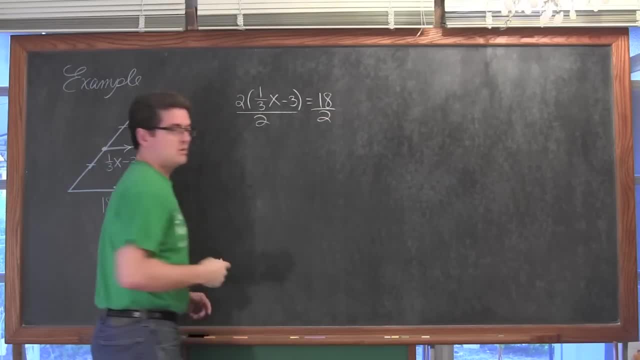 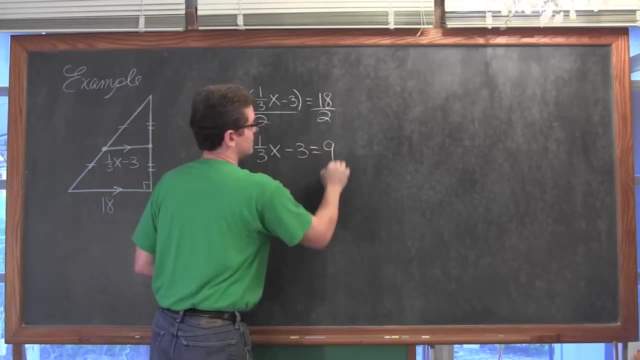 do that now and take this equation and divide it both sides by 2.. This may be unnecessary for how you set it up. I am just trying to teach you this material and help it make sense to you. So I am taking the 2 and dividing it from both sides, or again, just realizing. 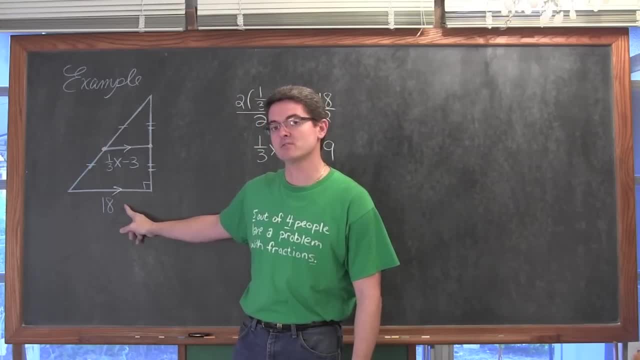 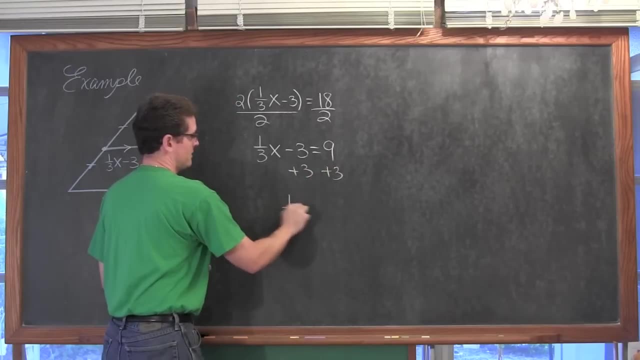 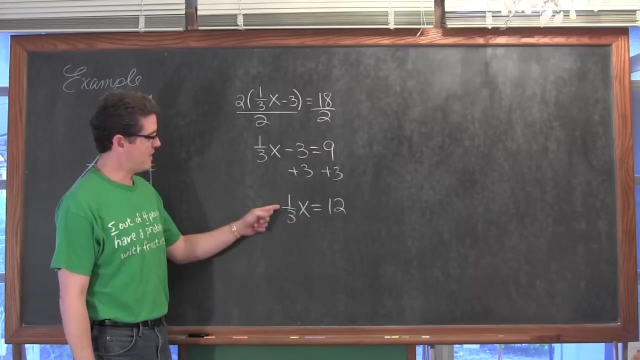 that this segment is equal to half of this side which it is parallel to. So we are going to finish solving this for x by adding 3 to both sides and get 1 third. x is equal to 12.. Now again, I have a fraction in front of my variable. A fraction simply means division. 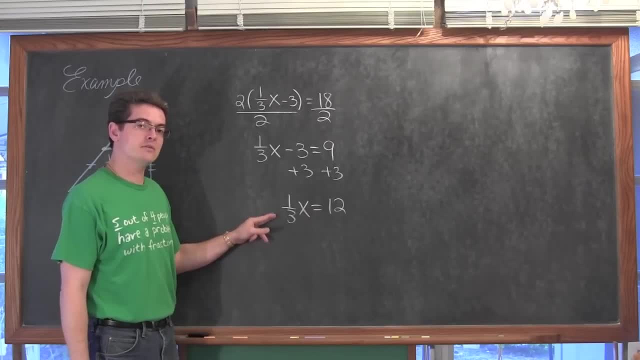 So I want to undo that division of 3.. Now I am going to undo a division of 3 by multiplying both sides by 3.. That multiplication of 3 and that division of 3 are going to cancel out. Or, since in the last video we took that entire. 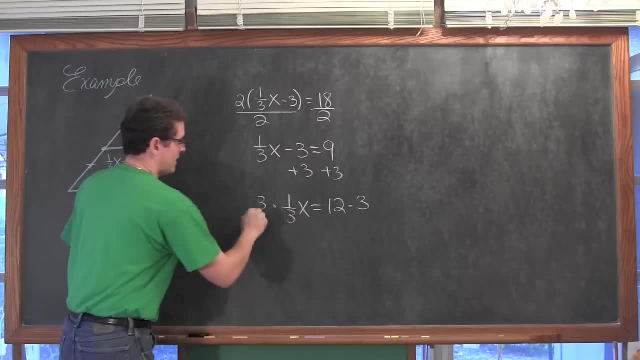 4 and divided it by 3, we are going to cancel out that division of 3.. So we are going to take that fraction and wrote it as a reciprocal. We flipped it. I can go ahead and put that over 1 and have the same thing that happened before. We have 3 over 3.. That is going to 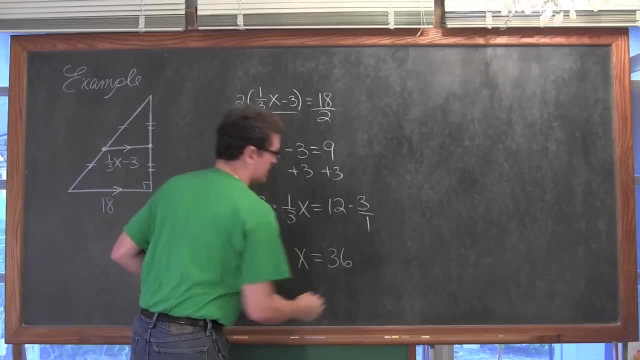 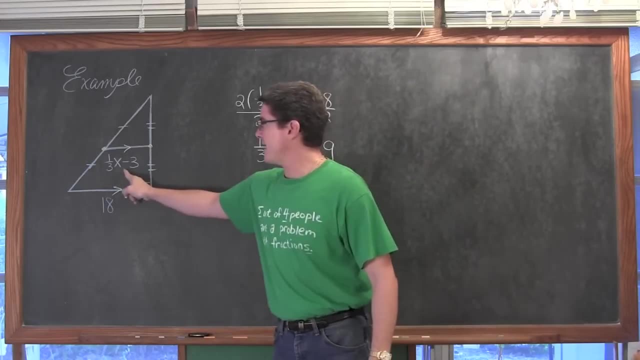 cancel out to be 1. We get x is equal to 36.. That is it, We are done. If you want to make sure that this is actually the right answer, of course we can take it back in here and plug it in and see what happens. You know, do a check. It is never a bad idea to make. 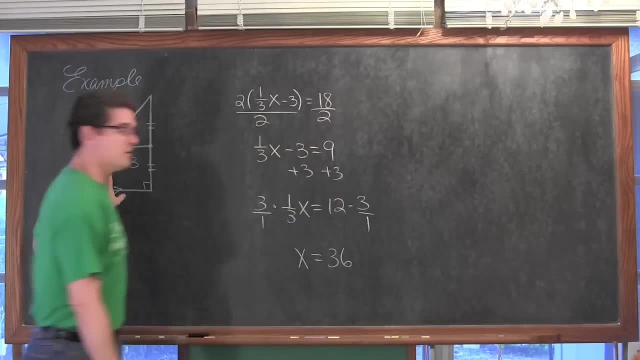 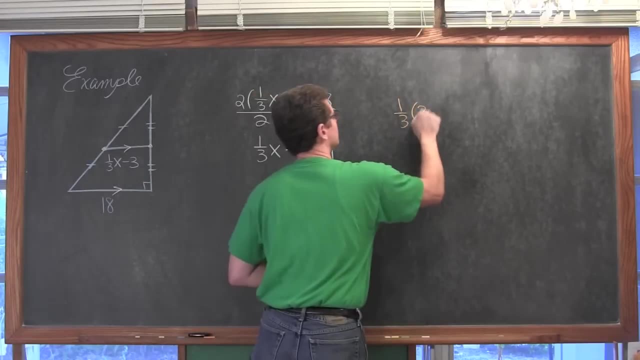 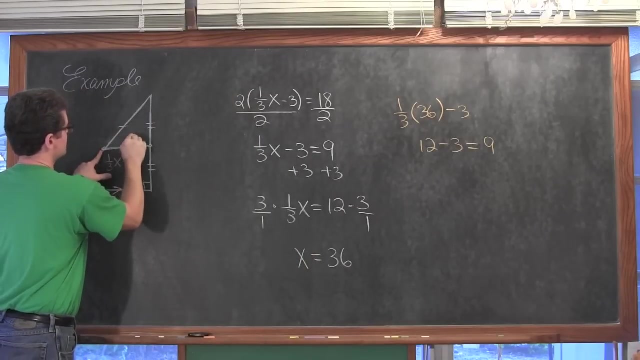 sure our own work is right. So we can take 1 third times x Minus 3.. So 1 third times x, which is 36 minus 3.. That is going to be 1 third of 36, is going to be 12 minus 3.. That equals 9.. Let's see A length of 9,. is that equal to half of the? 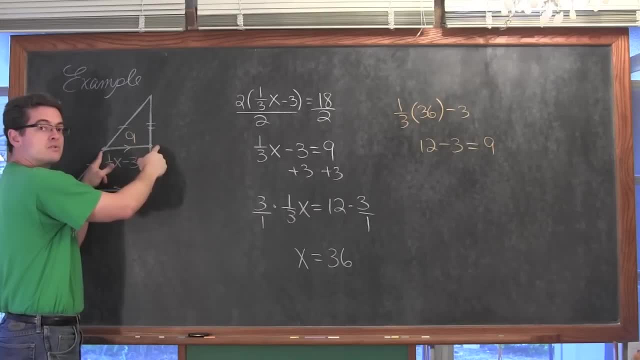 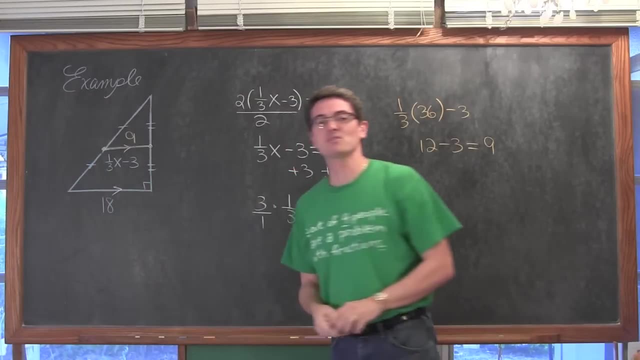 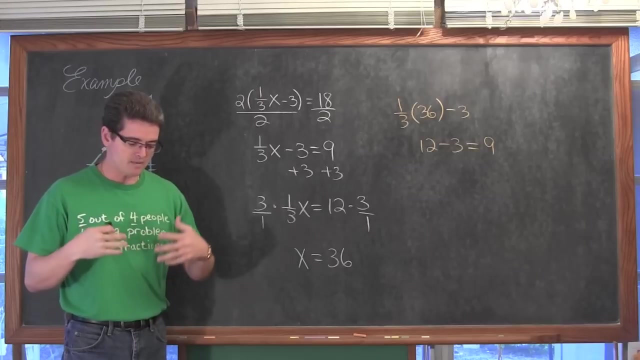 parallel side Is that segment connecting the midpoints of two sides of a triangle equal to half of the third side. Last time I checked that was correct. I have one more example for you. It is going to be a systems of equations So I will have to do a little bit of substitution method to 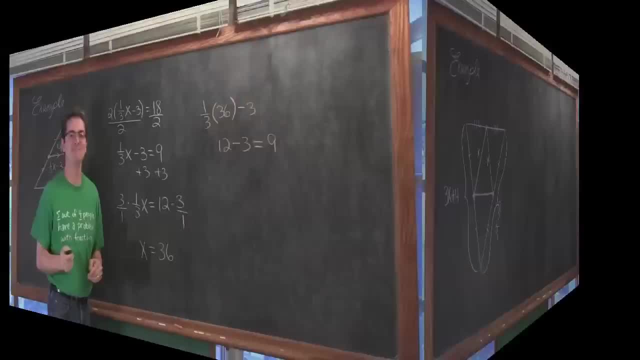 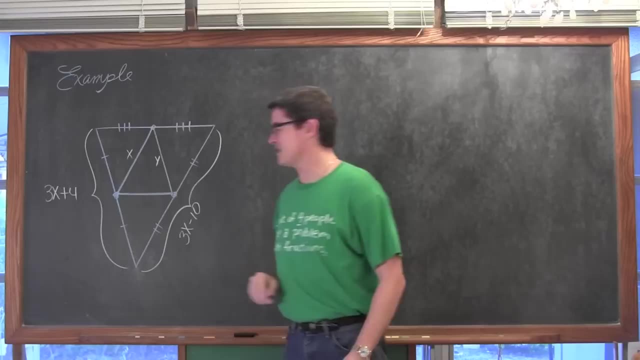 get those systems solved for and we will be done with this video. Thank you for watching again. Last example: We have a big old triangle and we have all three midpoints being marked. That means we have a lot of segments connecting the midpoints of the sides of a triangle. 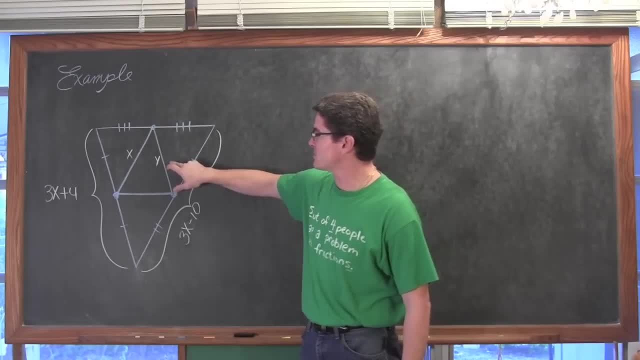 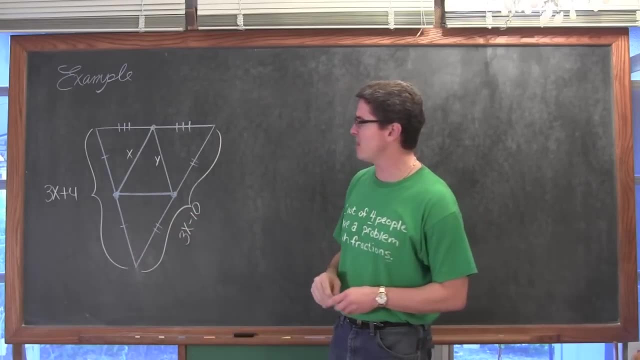 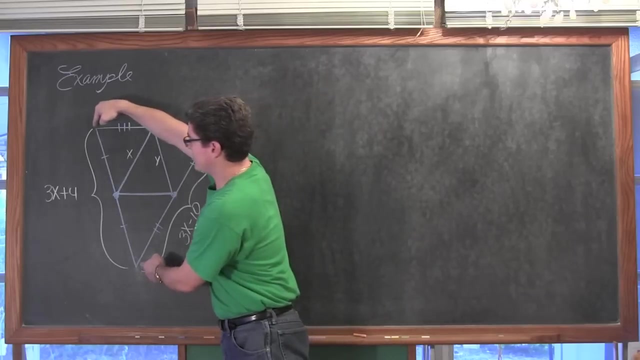 Which means that this blue line with the label of y on it is equal to half the length of the third side of the triangle, which it is also parallel to. But I don't even know that they are parallel. to do this problem, All I need to remember is that this segment is half the length of this segment I want to 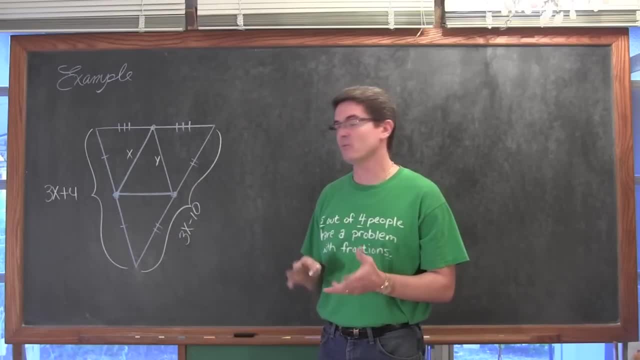 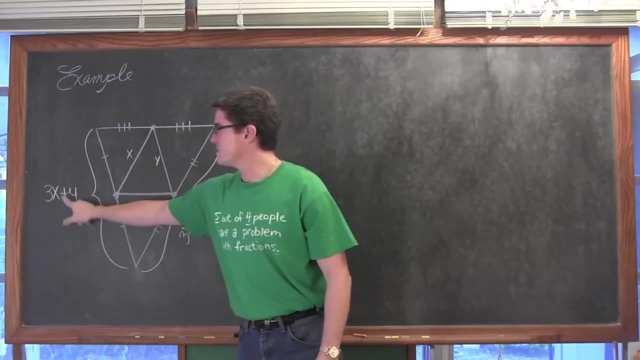 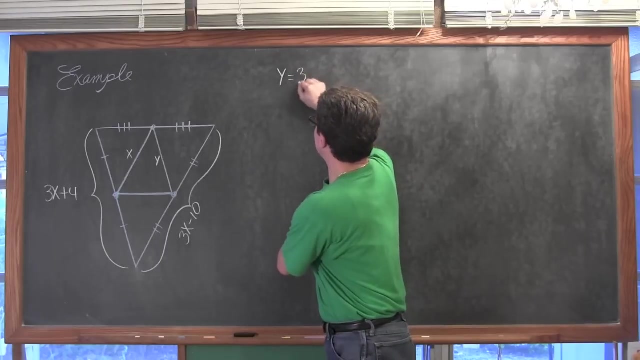 use the information on this diagram to solve for x and y. So when I set up my equations I need the two sides to be equal. So I want to relate this unknown value of y to this expression of 3x plus 4.. Now I can't just say that y is equal to 3x plus 4, because they are not equal. This. 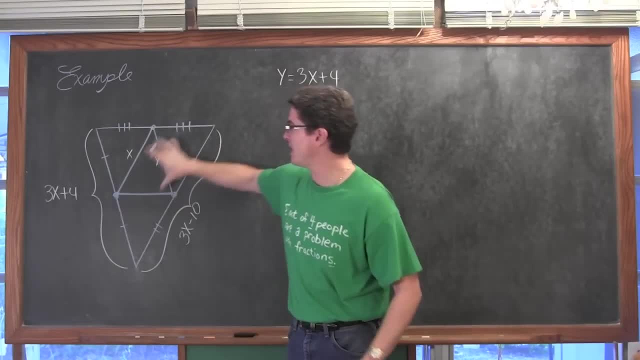 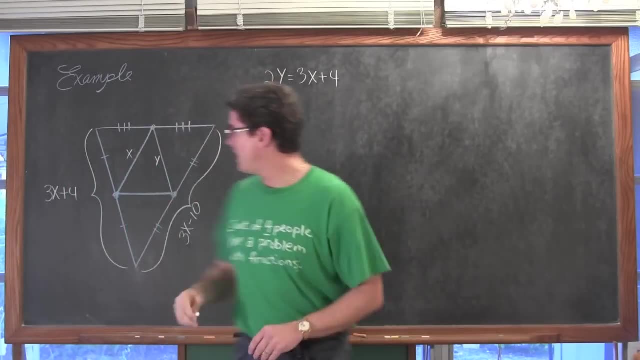 length is half of this length. So if I want to make them equal, I am going to take this and multiply it by 2. So we have: 2y is equal to 3x plus 4. We can set up another equation. 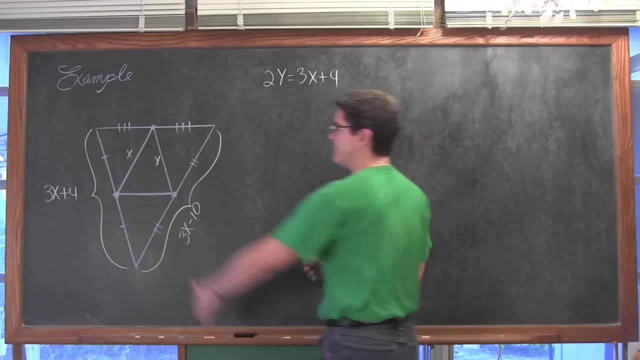 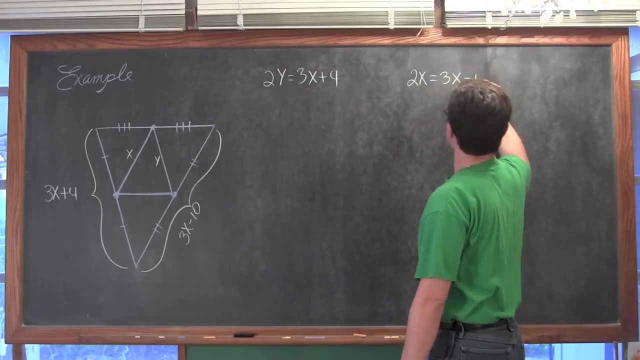 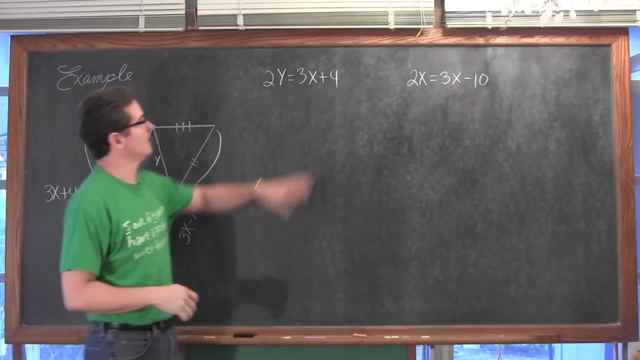 for x. This x is half the length. This segment connecting the midpoints is half of this third side. So I am going to take 2x and set it equal to 3x minus 10.. I need to take these two equations and use them together to figure out what both x and y are equal to. Well, I 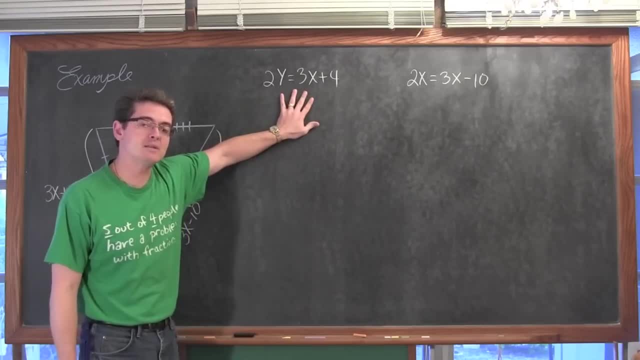 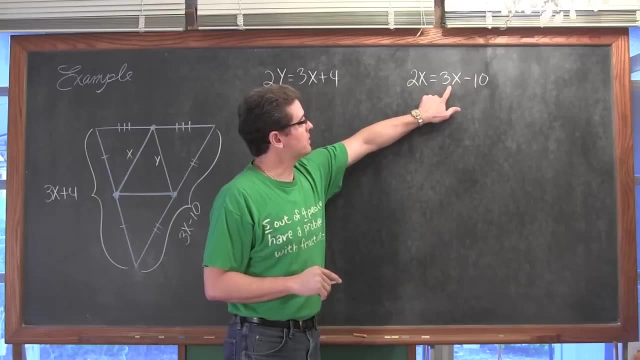 can't start off with this equation, because they have two variables in the same equation, which means I am not going to be able to solve for both at the same time. However, this equation only has one variable, So we are going to solve for x. There is nothing in there. I'm 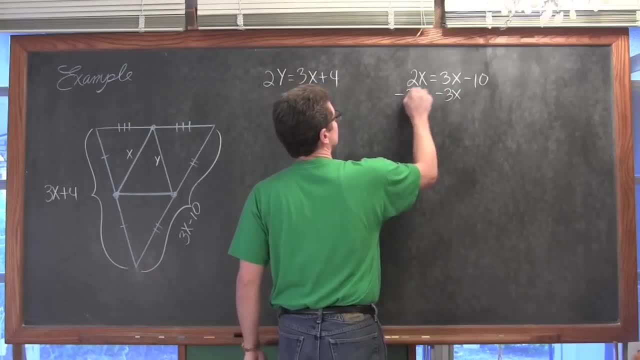 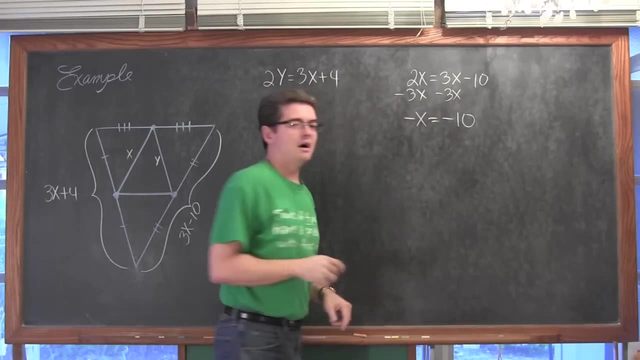 going to take 3x. We are going to subtract it from both sides, Get 2 minus 3, which is negative 1. So we have negative x is equal to negative 10.. I want to solve this for x. We do not have a variable to solve for until it is completely alone. That is including 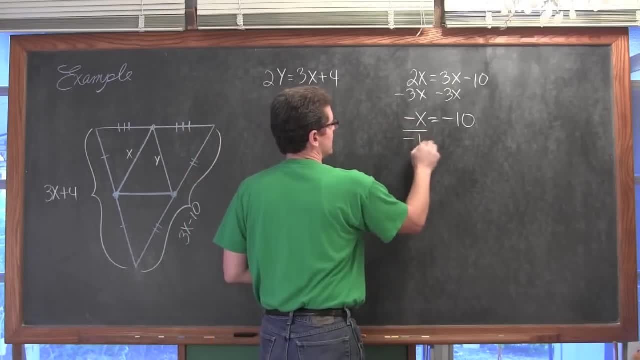 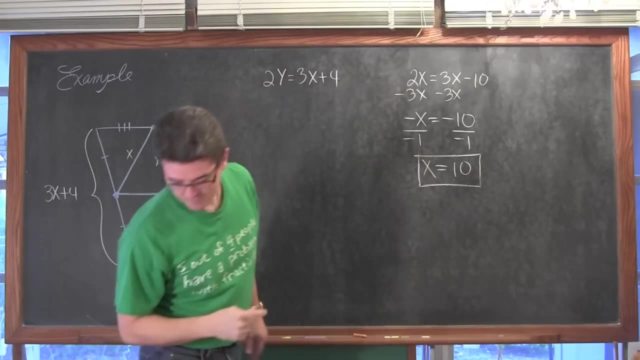 the negative that is in front. So we are going to get rid of that negative by dividing both sides by negative 1 and get x is equal to 10.. Let me just make sure I am not making mistakes here. Well, yes, it is 10.. 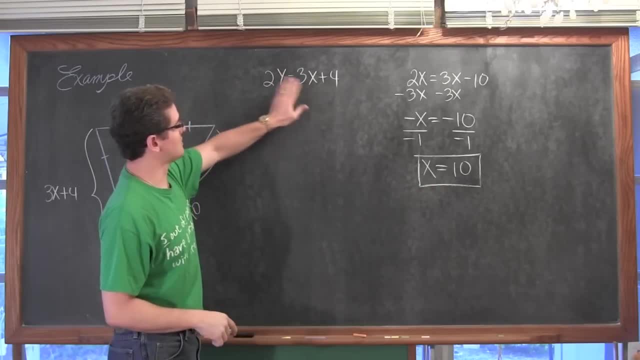 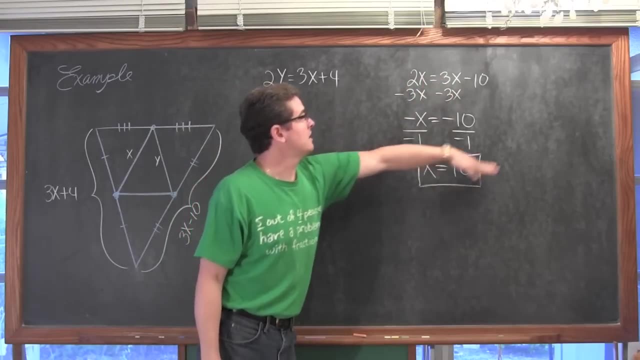 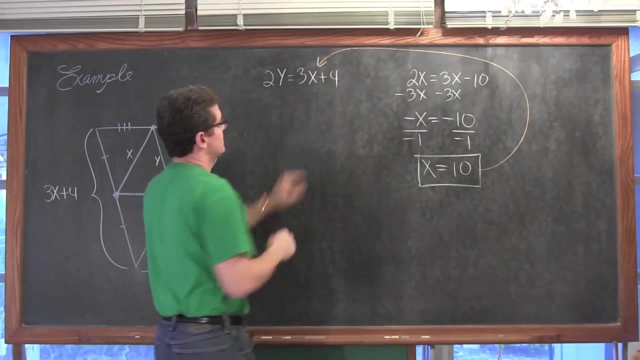 Ok, now that I have one of my two variables that are in this equation, I can use substitution to bring the information that we know from this equation into this one. So we are going to take this x value of 10.. We are going to bring it in and drop it in place of the variable. 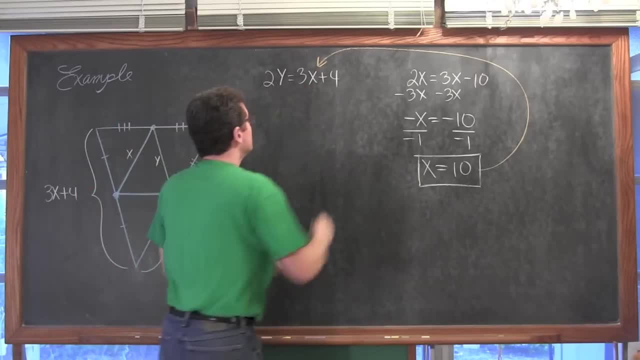 x and rewrite this equation, so there is only one variable left. So we are going to bring this down and we are going to have 2y equals 3 times 10 plus 3 times 10.. So we are going to have 2y plus 4.. We are going to, of course, need to follow the order of operations which 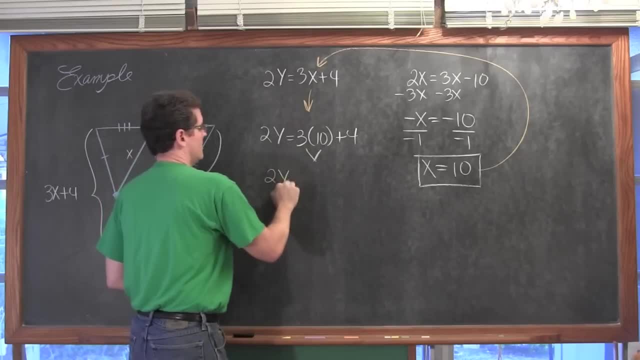 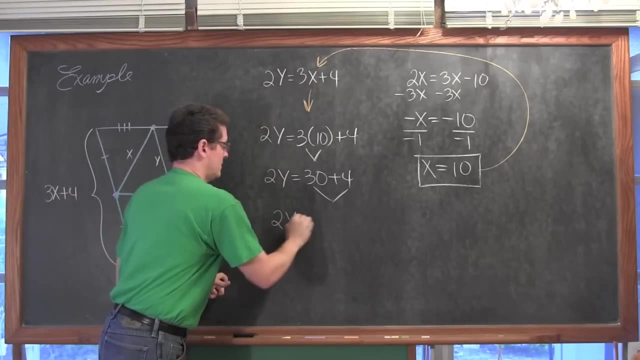 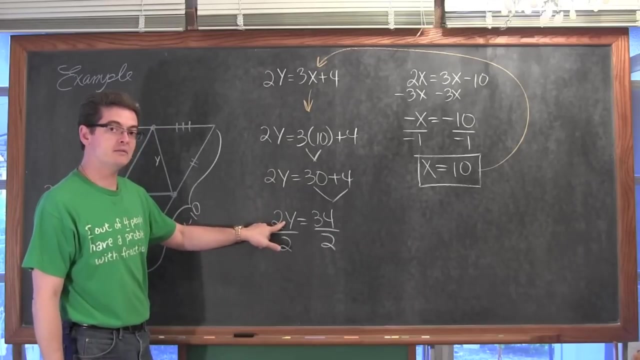 means we need to multiply and then add. So we are going to have: 2y is equal to 30 plus 4.. Continue adding like terms on the same side. We get 2y is equal to 34.. Divide both sides by 2.. We are now switching the math operation and doing the inverse math operation. 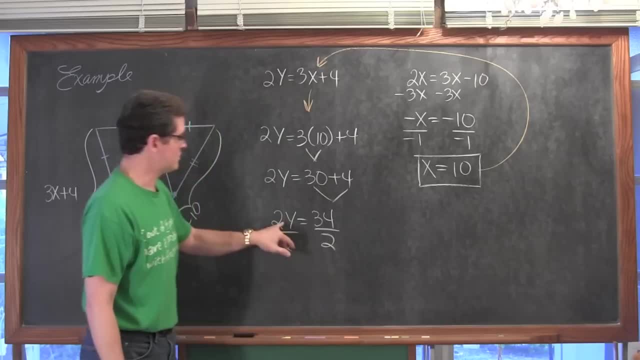 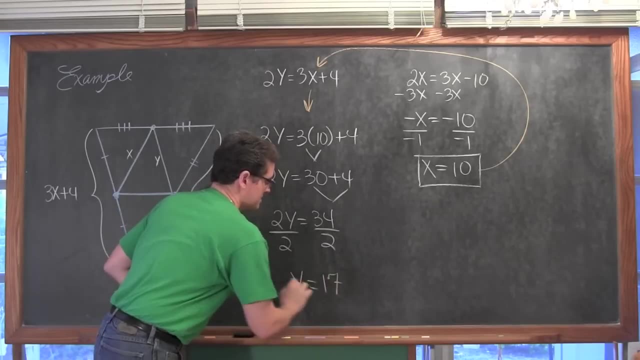 because I want to bring that 2 over to the other side of the equation, Which means I need to do the opposite of multiplication, Which is The final answer is going to be: y is equal to 17.. Now again, if I want to check these, 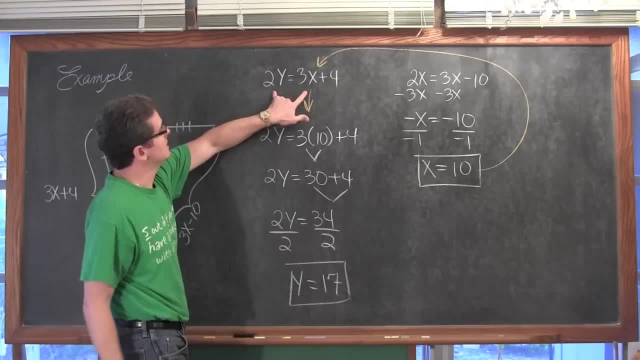 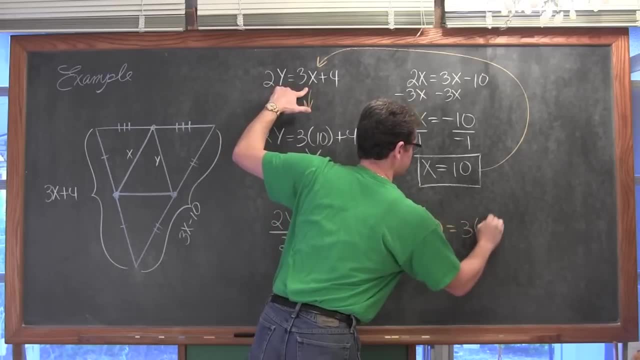 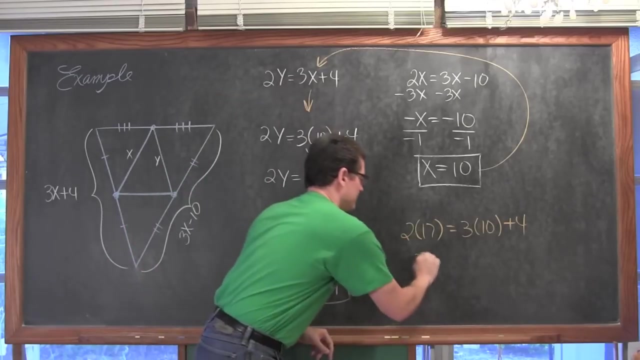 answers, I can take them and plug them back into these equations. Let's see here: Do we have: 2 times 17 is equal to 3 times 10 plus 4.. We have: 2 times 17 is equal to 34.. We have: 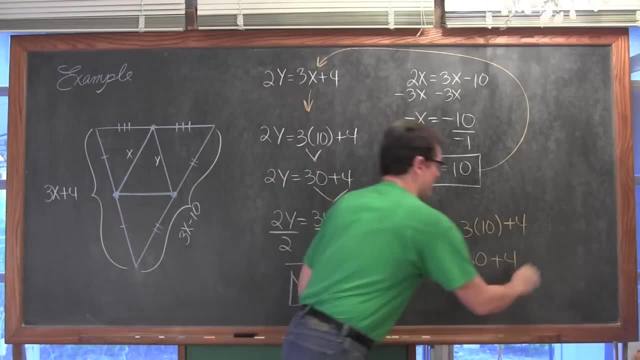 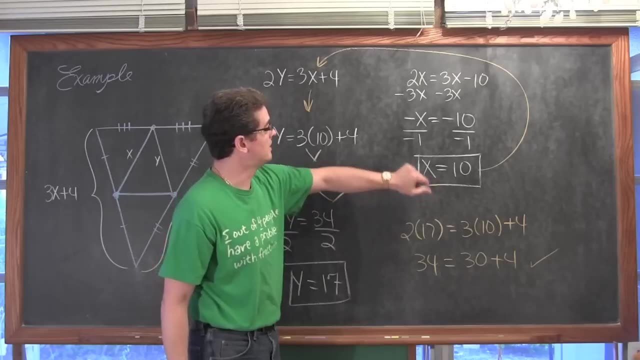 30 plus 4 does equal 34.. So I have gotten a couple of answers. I have plugged it back into one of these equations and made sure it actually works. I can take the value of 10 and plug it up here as well to make sure my answers work for both equations We have. 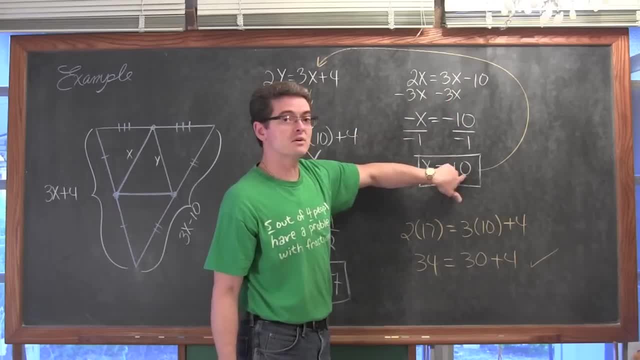 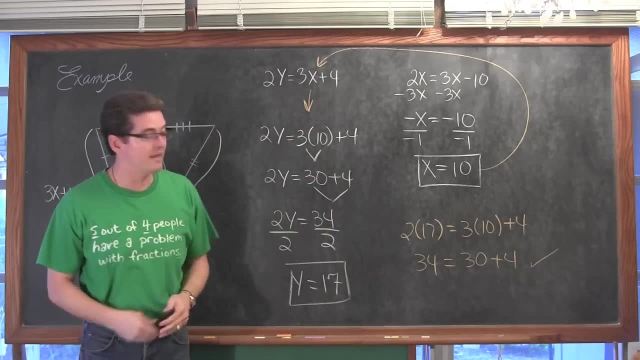 2 times 10 is 20.. We have 3 times 10, which is 30 minus 10, which is also 20.. So we have checked our answers out of both equations and that means I am done with this problem and I am done with this video. So I am Mr Tarrou BAM, Go Do Your Homework.